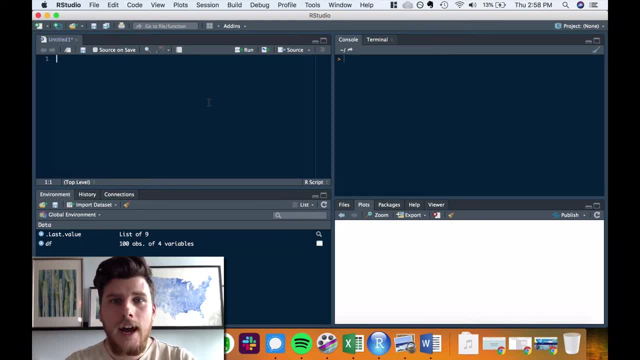 Hi, In this video, I'm going to show you how you can use color to map categorical variables in ggplot. Throughout this video, we're going to be working with the mtcars dataset. This is a dataset that has information on the number of different cars. 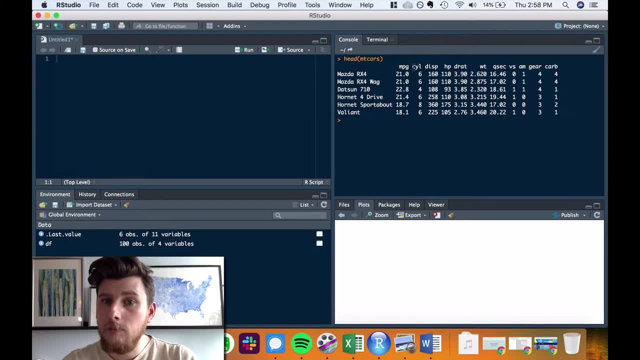 It talks about things like the miles per gallon for the car, the number of cylinders in the engine, the horsepower of the car and the weight of the car, among other things. Let's graph a simple scatterplot of this data. We'll be using the geompt function and we can map the weight variable to the x-axis. 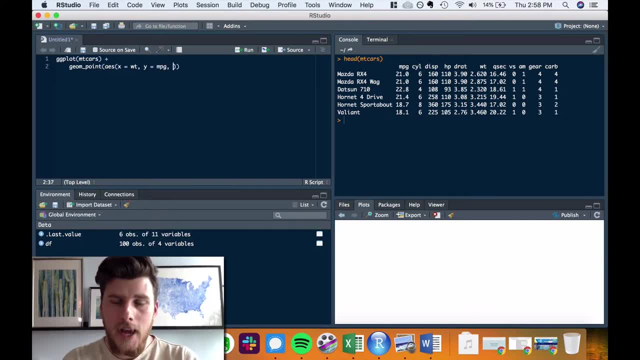 and the miles per gallon variable to the y-axis. I'm also going to show you here how you can map the engine cylinders, that's the cyl variable, to the gpl variable. To color, In this case, engine cylinders is a categorical variable in reality. 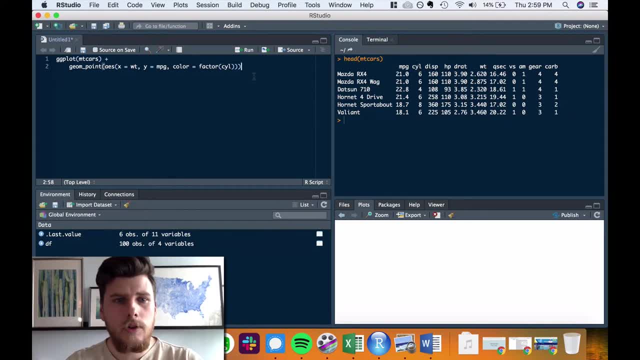 but it's recorded here as a numerical variable. So in order to force it to show up as a categorical variable, we're going to convert it to a factor, which will cause there to be only three levels in the dataset for four, six and eight cylinder engines. 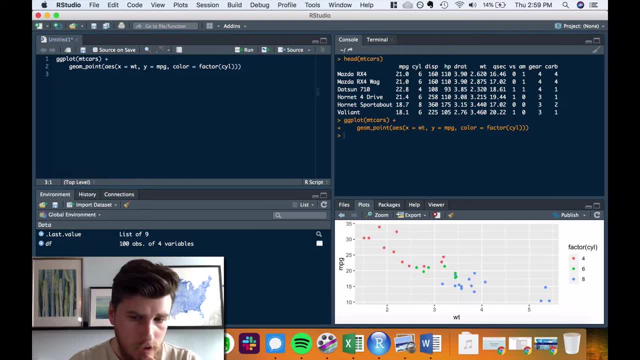 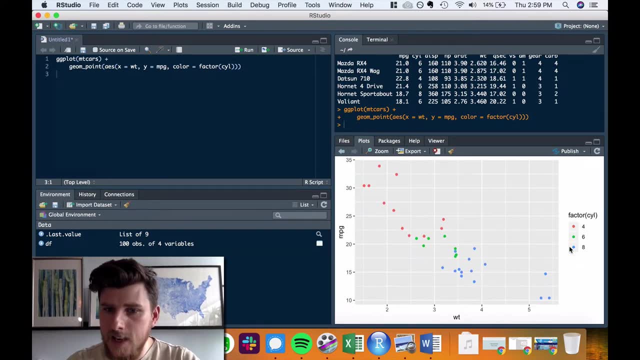 So let's take a look at how this looks in our data. Okay, so we have a nice scatterplot down here where each of the three different engine cylinders- four, six and eight- shows up as a different color in the scatterplot. 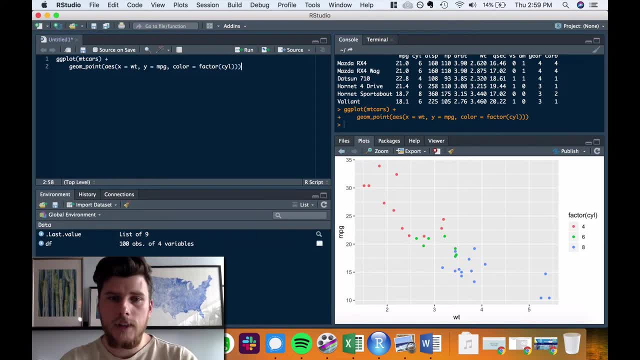 So this is nice, but I want to show you specifically how you can actually change the colors of these individual points. The way that this works is you first want to define the colors that you're going to map to, and then you create- I'm going to create here- a vector. 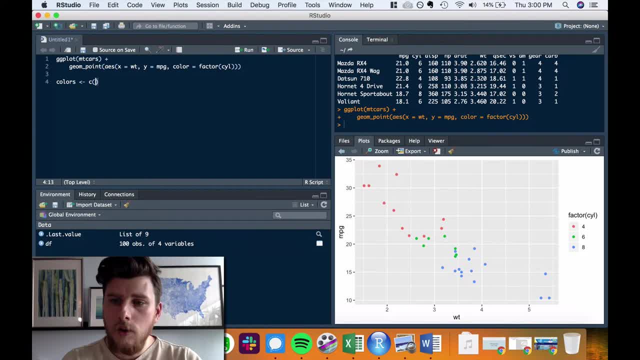 I'm going to call it colors, but you can call it whatever you want, And for each of the values in your underlying dataset, that's four, six and eight, you want to map them to a specific color within your vector. So, again, you can put any single color that you'd like in here.